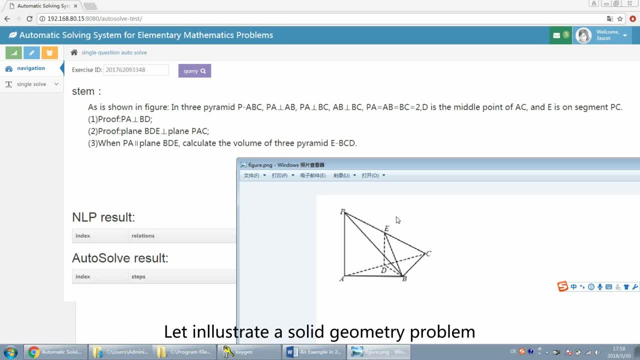 Let illustrate a solid geometry problem as an example to demonstrate the whole autosolving process, As is shown in the figure in three pyramids: P A, B C. P A is perpendicular to A B. P A is perpendicular to B C. 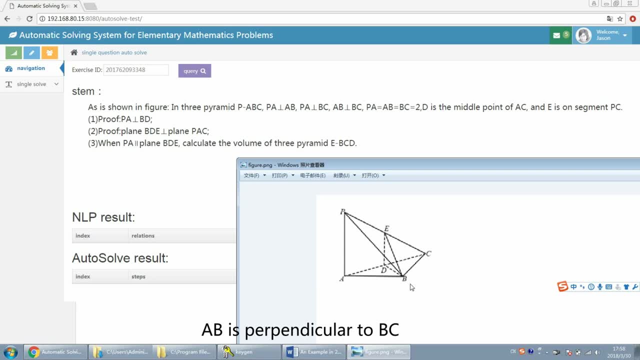 A, B is perpendicular to B- C. P, A equals A, B equals B, C equals 2.. D is the middle point of A, C And E is on the segment P- C. The question need us to solve three. problem Number one: Proof. 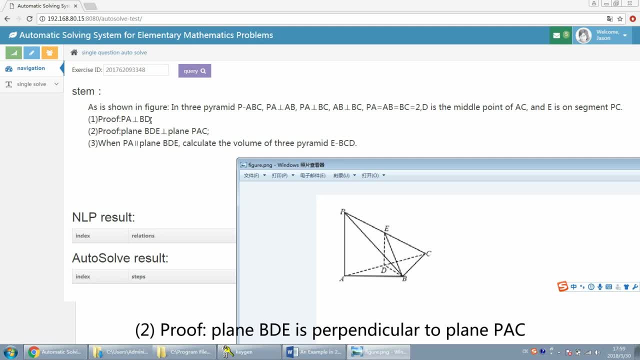 P A is perpendicular to B D, Number two. Proof Plan B D E is perpendicular to plan P A C, Number three. When P A parallel to plan B D E, Calculate the region Of three pyramid: E, B, C, D. 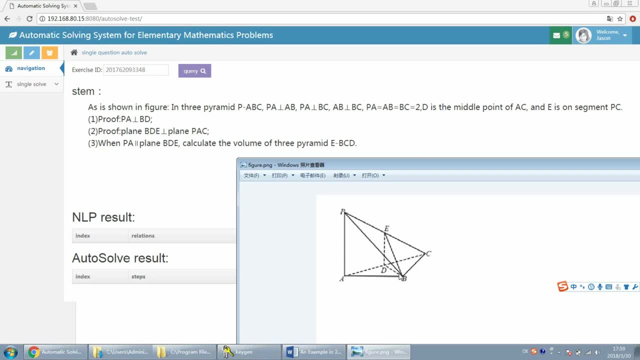 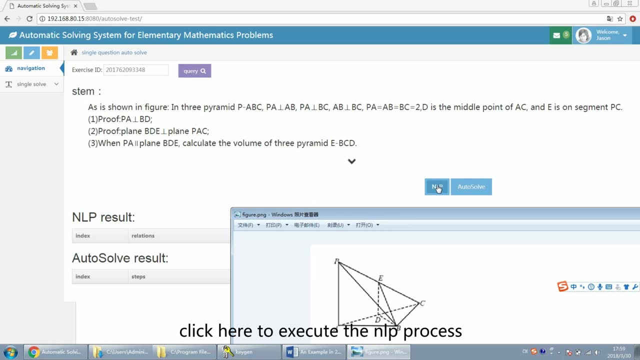 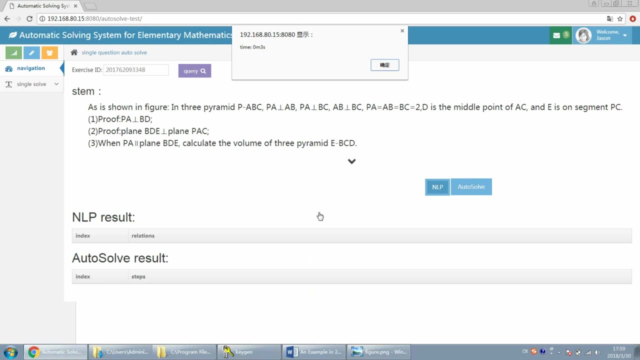 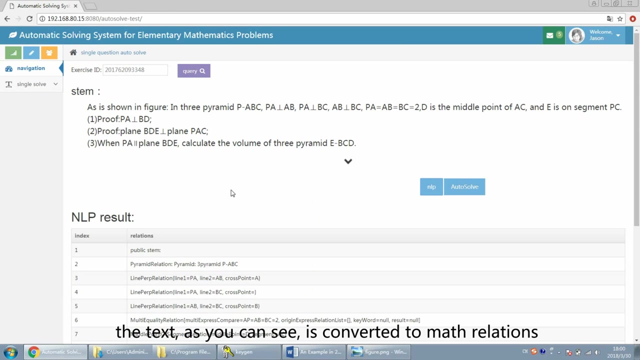 Next We will talk about the solving process, The first step: Click here To execute the NLP process. The test, as you can see, Is converted to math relations, Which is represented in first order Predicate logical forms Such as: